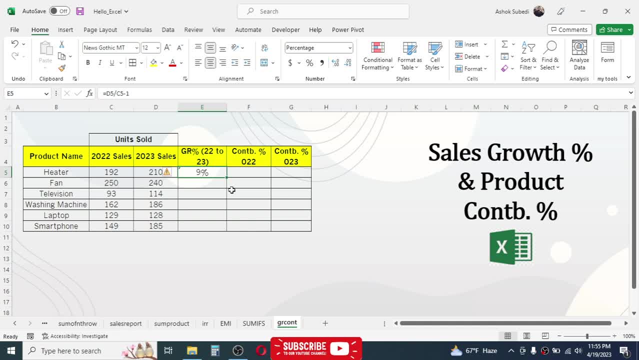 to 2023 for the product heater. If your result is displayed in number formatting in this way, you can simply change this into percentage formatting by clicking on the percent icon here and it is given. and if you want to display the digit after the whole number, then you can click on this increase. 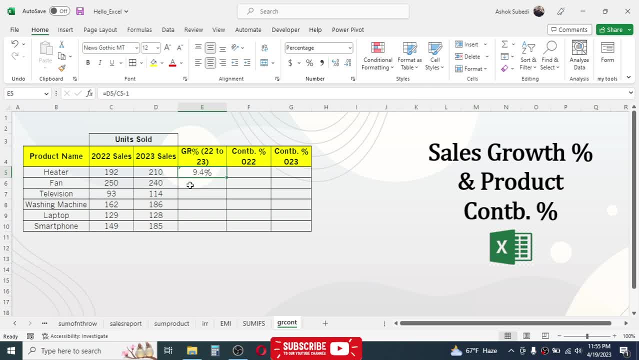 decimal icon And here you can see it is given in the decimal format. Now you can simply drag this till the last product and here you can see all the growth percentage are calculated. This product has the degrowth of four percent. The negative- some numbers are in negative Negative means there is 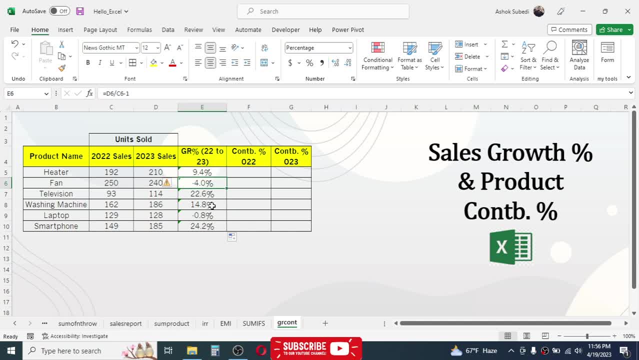 degrowth and positive means there is growth. So this is the way we calculate growth percentage. The second formula we can use here is MDF, Deleting this formula and showing you the next formula, which is equal to open the bracket. then click on the 2023 sales minus 2022 sales. close bracket. then divided by 2022 sales. 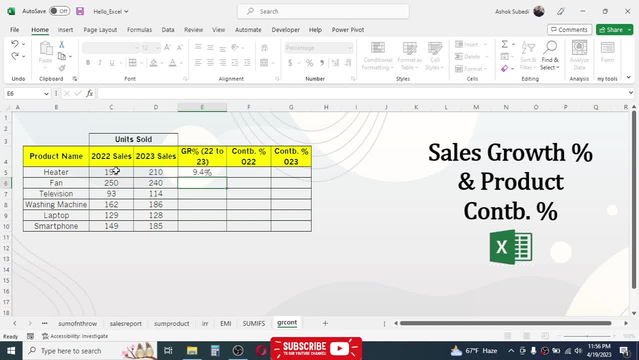 So this is also the formula for calculating growth percentage. Here also you can see the same result. This formula means the current year sales minus last year sales divided by last year sales, Which calculates or which gives us the growth percentage, As you see, here you can click. 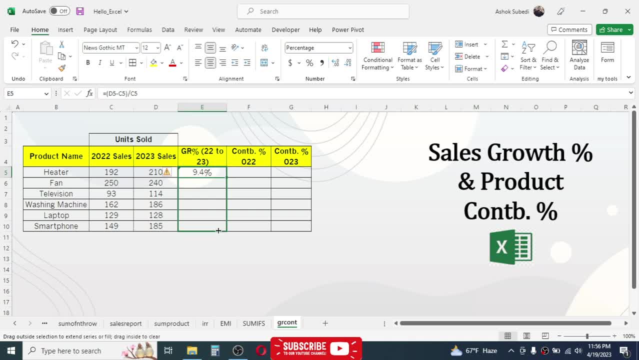 on this plus button and then drag it for other products, and here you can see the growth is calculated by this second formula also. The next one we are going to calculate here is the product contribution percentage. and to calculate the contribution, first of all here we need to calculate the grand total. 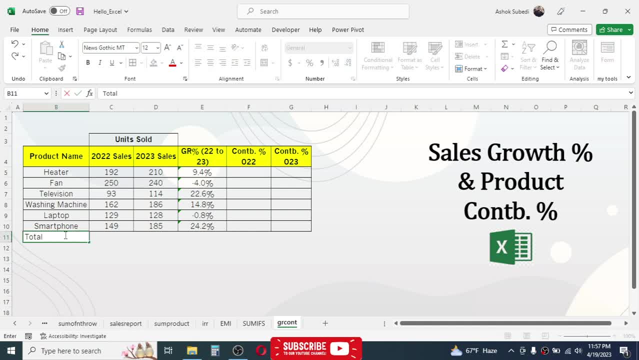 So here I am calculating the total You need sold here by using formula. Here, in these two cells, I am calculating the total by using sum function and here you can see this is the total sold quantity. and based on this total quantity and individual quantity we will calculate the growth percentage by using a very simple excel formula, which is: 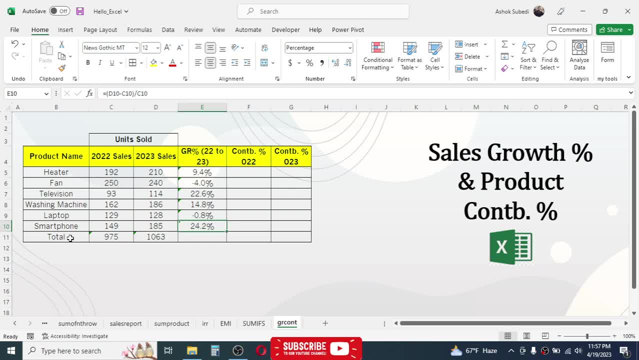 here I am going to show you the formula for calculating contribution percentage. Click on the cell, then press equals. Click on the individual products sale in the 2022 year divided by then we have to click on the total. Individual divided by total gives you the contribution, and here, in this case, we need. 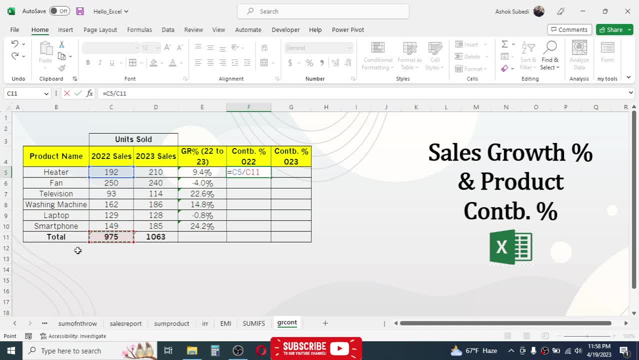 to fix this C11 cell, because when we drag the formula down, in that case this cell should move down, But this cell should be fixed here. That's why we need to give the dollar sign before C and before 11. here We can do this by simply pressing the F4 key in the keyboard, which will apply the dollar. 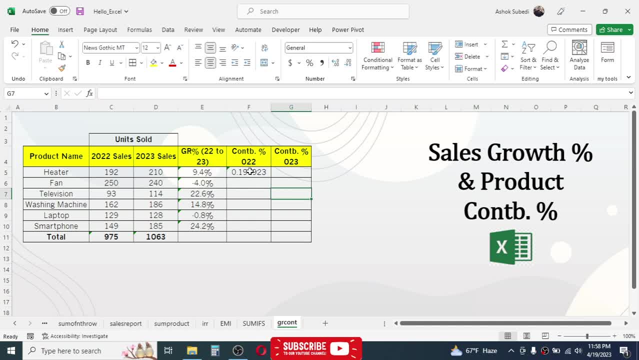 sign here, And here you can see it is the contribution is calculated and we have to convert this into the percentage formatting by clicking on the percent icon. Now you can see the contribution of heater to the total, So we have to convert this into the percentage formatting by clicking on the percent icon. 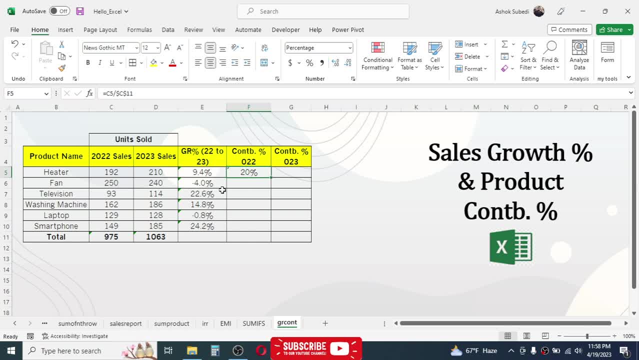 So the total sales is 20% in the year 2022.. You can now drag this till the last product and all the products contribution is calculated. The total is 100% and this is the individual contribution. The highest contributing product is fan, which has the contribution of 26%. 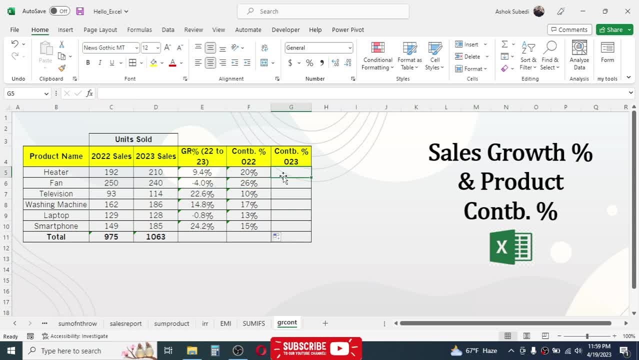 So in this way we calculate the contribution. Similarly, here also we can use the same formula equal to, then click on that 2023 sales And here you can see that the total sales is 20%, And here you can see that the total sales is 20%. 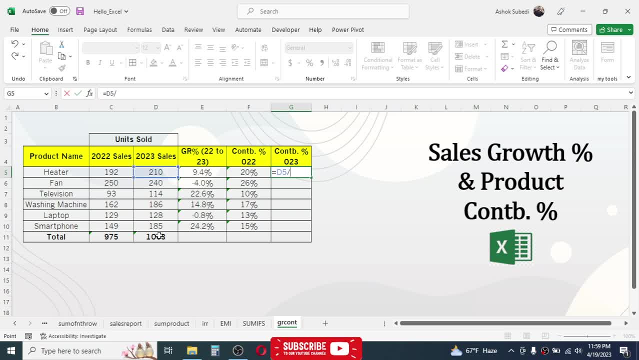 And here you can see that the total sales is 20%. And here you can see the fun fact of that: the total sales has increased successfully by making some contributions to 23%, Just by clicking OK. this will clearly show that the contribution is calculated here. 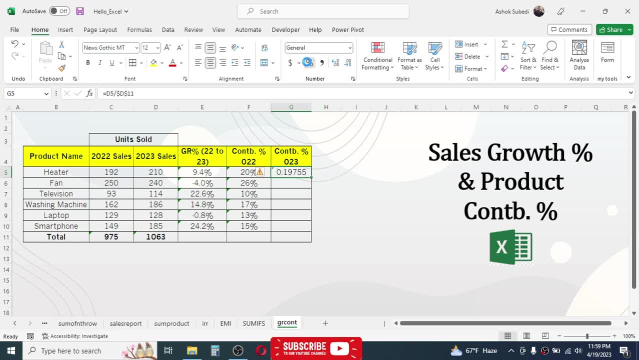 So now, if we mix all 2.. Thus we come up with the total sales In numbers, the total 잘못ed on the charge, context and quienes qui font. So here the contribution hurdle is already calculated. Moving on to value, questão one which is totally easy to compute. 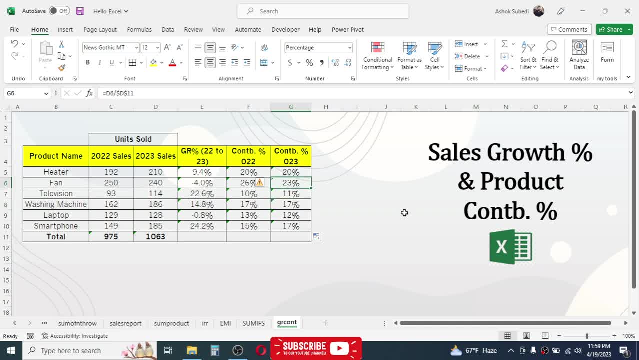 This is a graph we are looking for and you can simply drag the number for rank variable to this bar. we will get the value flavor value of 26.. Something like垧 in 2D value value value of 26 check function is also shown here.